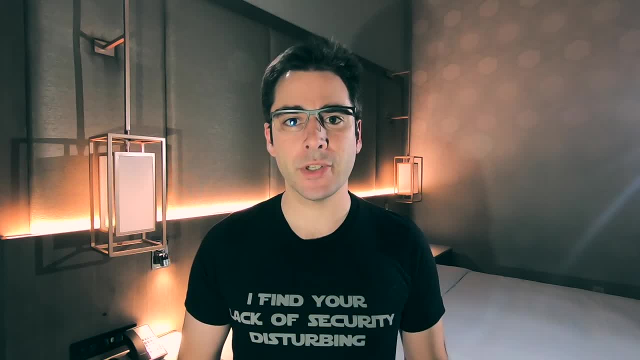 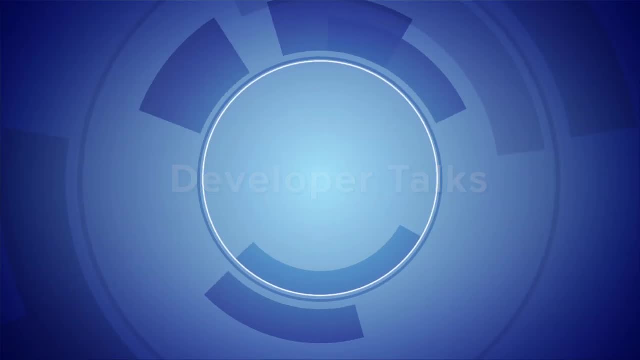 Hi, I'm Aaron Parecki. I'm at a hotel in Los Angeles right now, so I figured this would be a good time to explain a little bit about OAuth access tokens. So what are OAuth access tokens and what exactly are they for? Well? 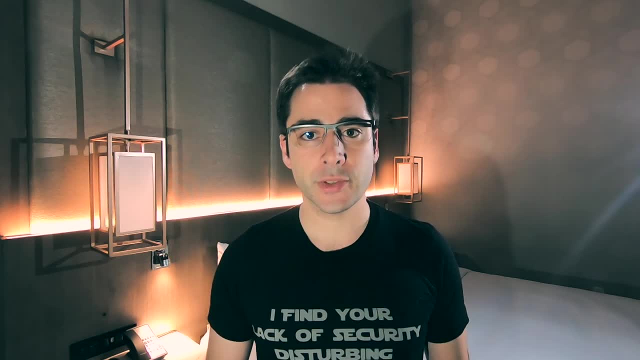 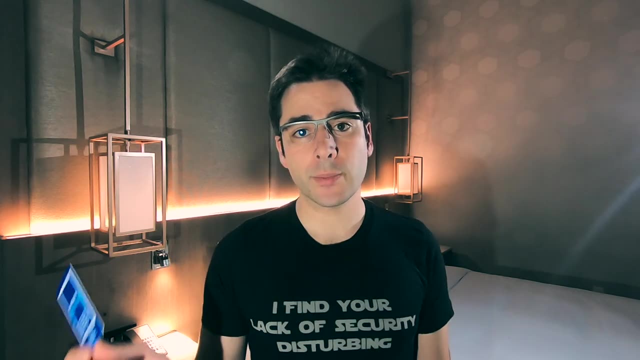 when I got to the front desk of this hotel, I went and I checked in. Pretty straightforward, exchange right. I showed my ID and I give a credit card and they give me back a key card. I then take this card and I walked up to the door of my hotel room and I swiped it on the door. 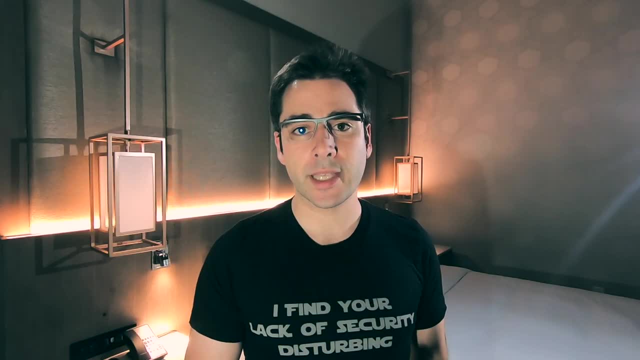 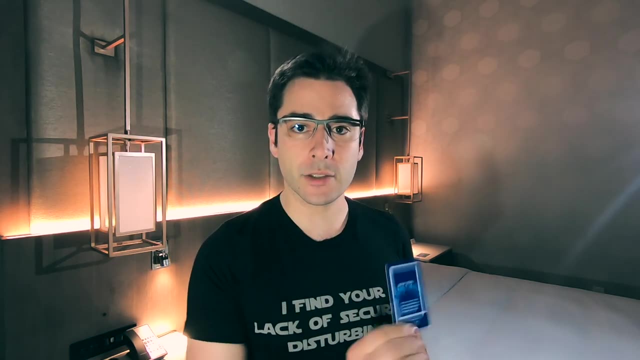 Of course the door let me in. So this hotel key card is like an OAuth access token. An access token just says whether or not the bearer of the token is allowed to access the thing they're trying to access, In this case the hotel room door. The door doesn't care who I am. 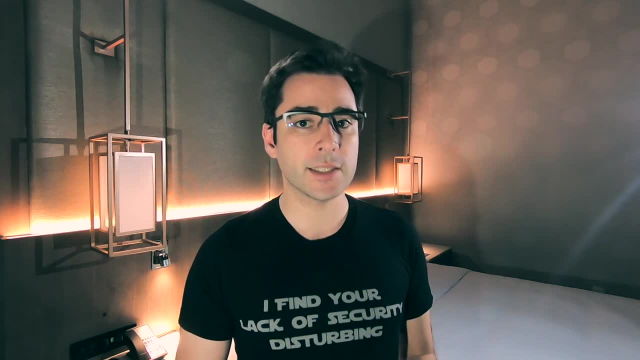 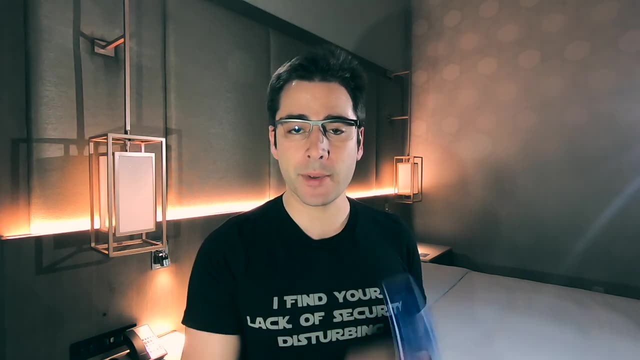 The door doesn't need to know my name or any unique identifier. It just needs to know whether or not this card is allowed to access this door at this time. This card doesn't have my name in it. It doesn't have my payment information in it. It just says that it can access this door. 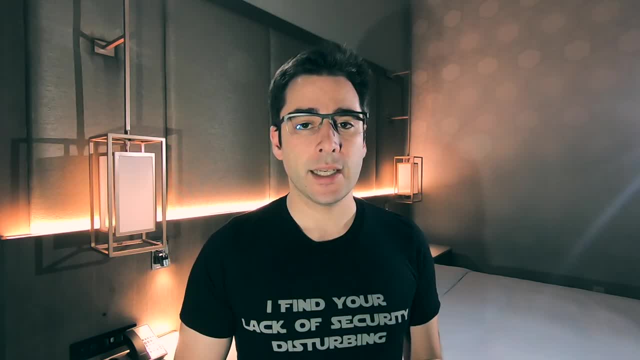 So an OAuth access token is exactly the same thing. The access token doesn't even necessarily have to have a user ID in it. All it needs to encode is whether or not the thing that has the access token can access the API, And that's why it's called a bearer token- The bearer of. 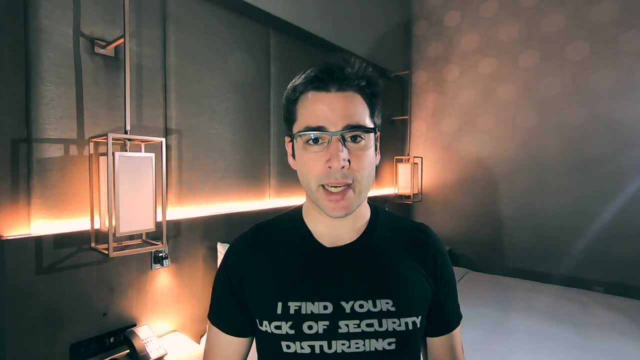 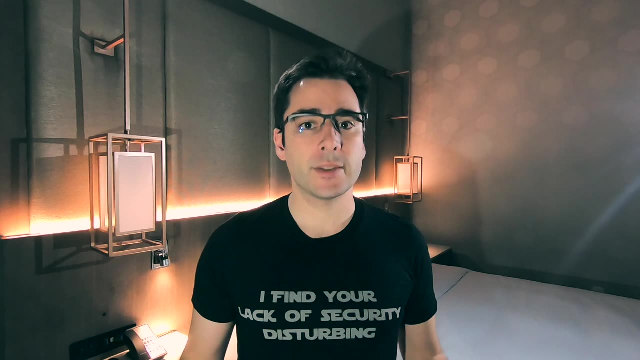 the token can access the API. Now you might be wondering: doesn't my API need to know what user this access token belongs to? Well, it may or may not Depends on your API. Of course, most APIs that deal with user information or storing resources for users they don't. But if you have an API that has a user ID in it, you might want to store the token in it. So, of course, most APIs that deal with user information or storing resources for users- they don't need to have a user ID in it. It just depends on your API And that's why it's called a. 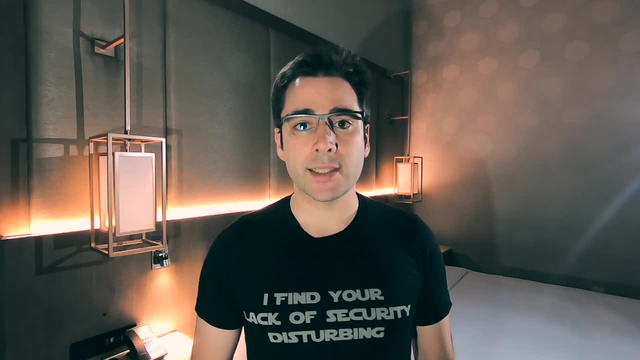 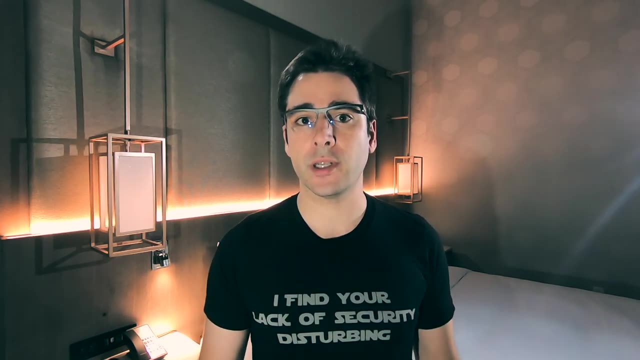 resources for users do need to know who the user is, in which case that access token might actually have a user ID encoded in it. But as far as the thing using the token is concerned, it doesn't care about whether or not a user ID is encoded in the access token, Just like my hotel key card. 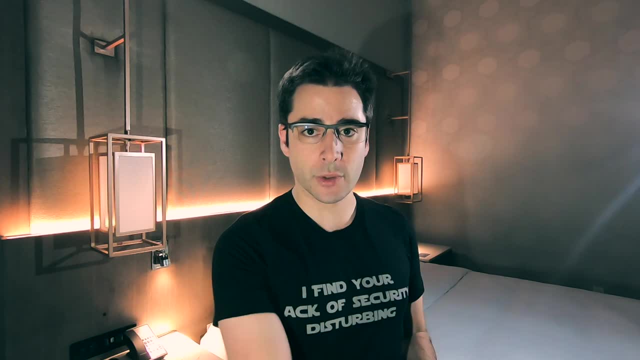 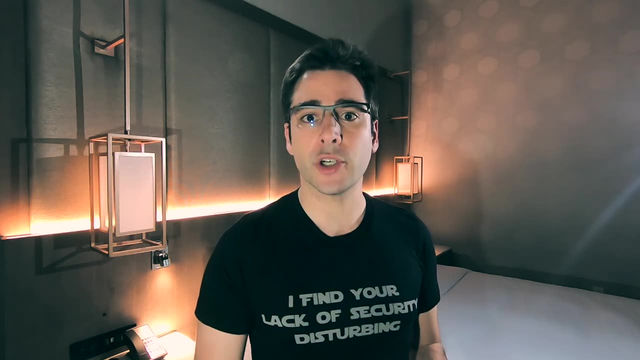 When I, in this analogy, the app presents the token to the door, I don't care what's in it. All I care is that it works. So I'm just going to take this key card, swipe it at the door, hope the door opens. Just like in an application, I'll take an access token, present it to the API.